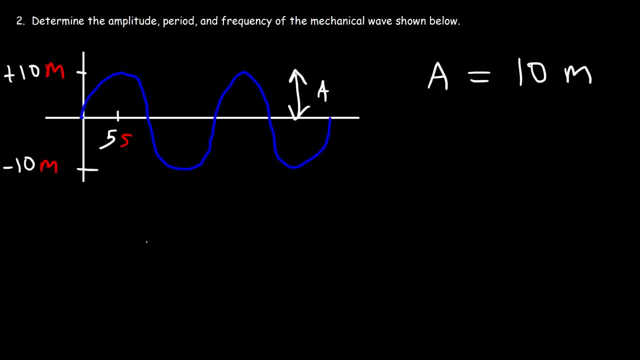 what about the period and a frequency of the wave? The period is the time it takes to make one complete cycle. So notice that the five seconds corresponds to the first quarter of the cycle. So at the second quarter, which is here, it's going to be 10. 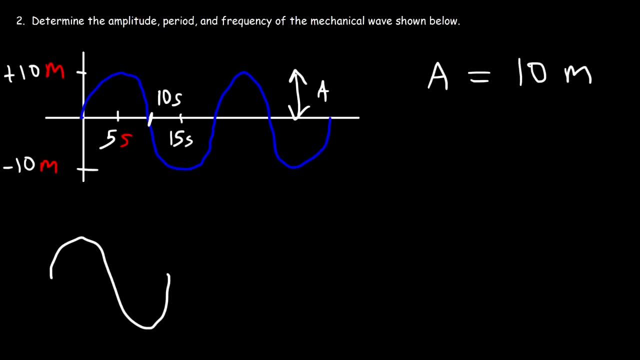 seconds. At the third quarter it's 15 seconds and at the full cycle, at the end of it, it's going to be 20 seconds. So the time it takes to make one complete cycle is 20 seconds. The frequency is 1 divided by the period, so it's going to be 1 over. 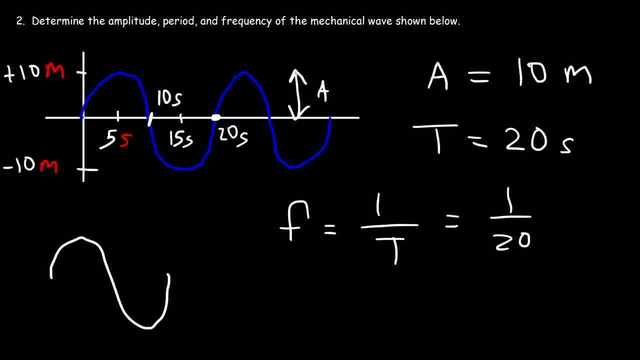 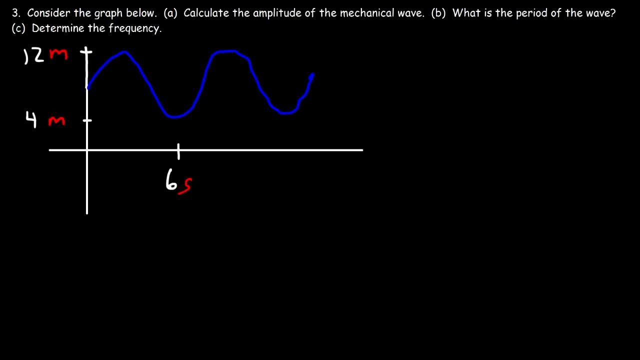 20.. So 1 over 20 will give us a frequency of 0.05 Hertz, and so that's the answer for this problem. So here's another example: Go ahead and calculate the amplitude of this particular mechanical wave. To calculate the. 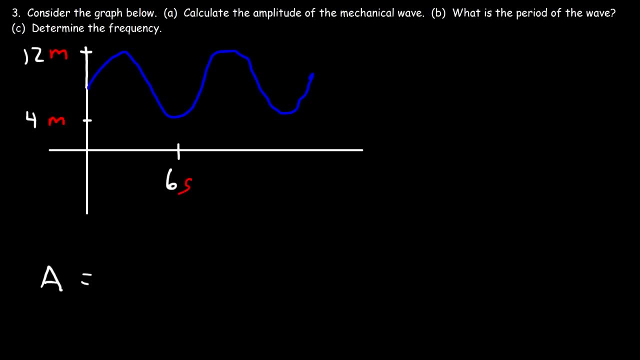 amplitude. it's going to be the difference between the highest value and the lowest value divided by 20.. So let's say H is the highest value, L is the lowest value, and so it's going to be 12 minus 4 divided by 2.. 12 minus 4 is 8.. 8 divided by 2 is 4.. So the amplitude in 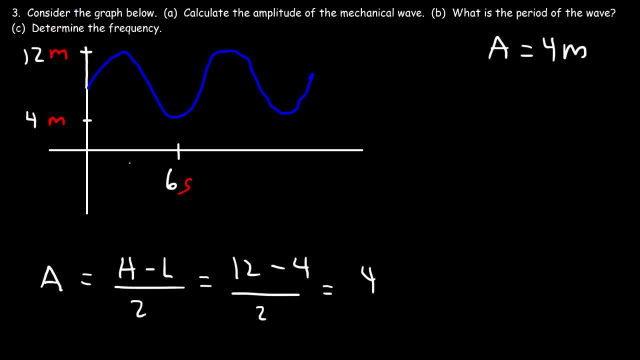 this example is 4 meters. Now the midpoint between 4 and 12 is 8.. If you add 12 plus 4, you get 16 divided by 2. That's 8.. And, as I mentioned before, the amplitude is the distance between the centerline and the highest point. So 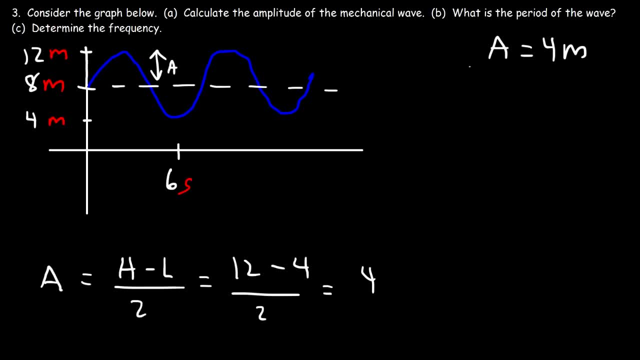 12 minus 8 is 4, and that will give us the same answer. Now, what is the period of this particular wave? So notice that the 6 seconds corresponds to 3 fourths of a cycle which would basically stop here at the bottom. So if we divide it, 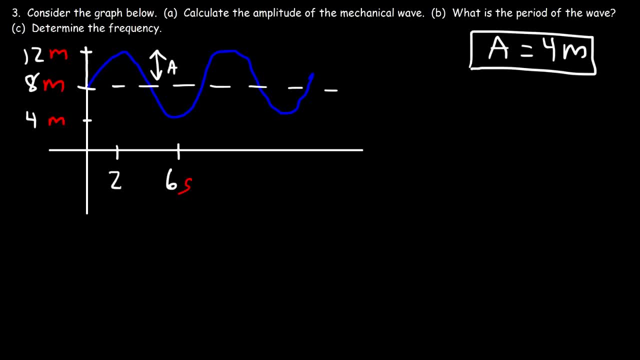 by 3,. 6 divided by 3 is 2.. So the quarter cycle would be at 2 seconds, the half cycle would be at 4, and so a full cycle would be 8 seconds. Therefore, the period is 8 seconds. 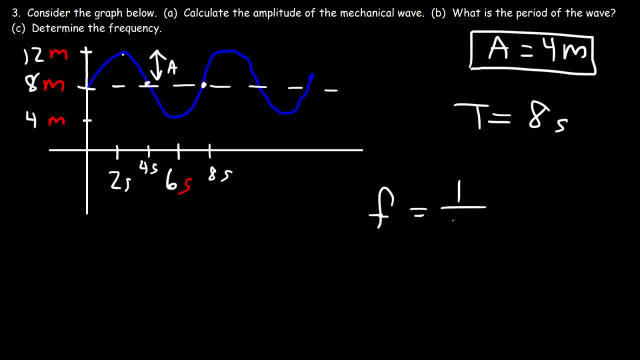 And now we can calculate the frequency. So the frequency is 1 over the period, so that's 1 over 8 seconds, and 1 over 8 will give us the frequency of 0.125 Hertz. And so that's how you can calculate the amplitude, the frequency, the wavelength. 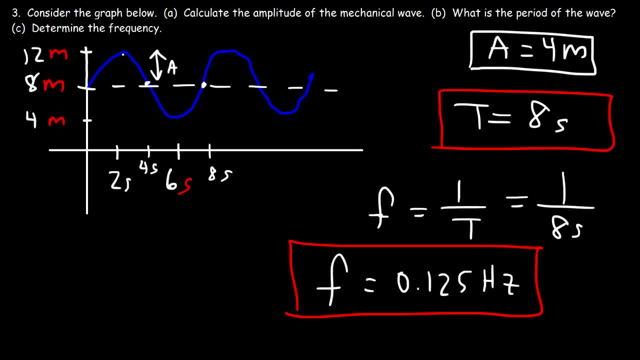 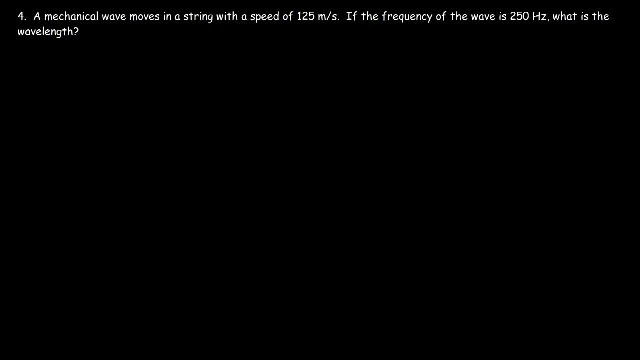 and the period of a mechanical wave, represented by a graph Number 4.. A mechanical wave moves in a string with a speed of 125 meters per second. If the frequency of the wave is 250 Hertz, what is the wavelength? So how can we find the? 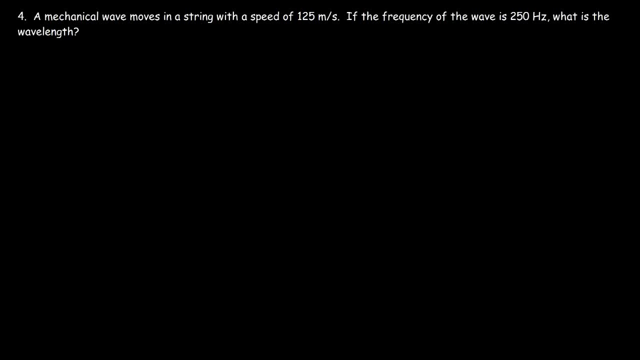 answer for this problem. The speed of a wave is equal to the wavelength times the frequency, And so the wave speed is 125 meters per second. We're looking for the wavelength, and the frequency is 250 Hertz. So to calculate the wavelength, it's simply the wave speed divided by the frequency. 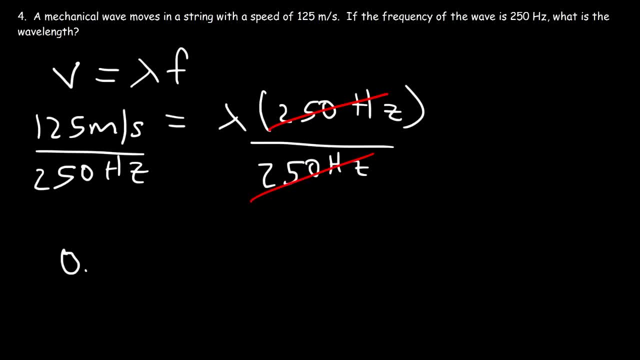 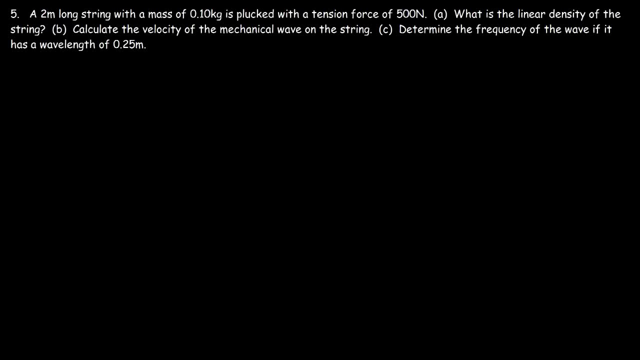 So 125 divided by 250 is 0.5.. So it's 0.5 meters per second. So the wavelength is 0.5 meters per second. Number 5.. A 2 meter long string with a mass of 0.10 kilograms is plucked with a tension. 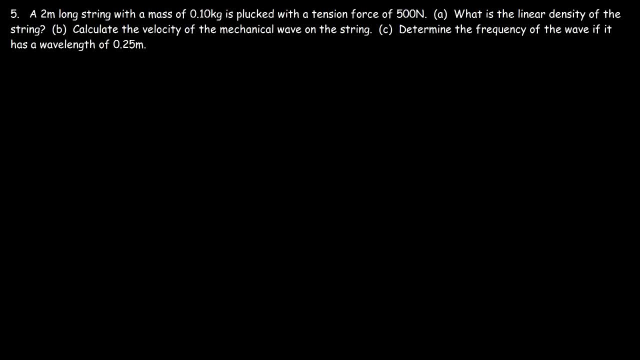 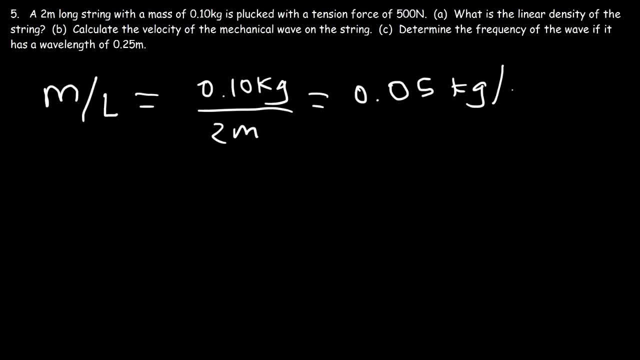 So 0.10 divided by 2 will give us 0.5 meters. So 0.10 divided by 2 will give us 0.05 kilograms per meter. Now let's draw a picture. So let's say, if we have two boundaries and a string is in between them, 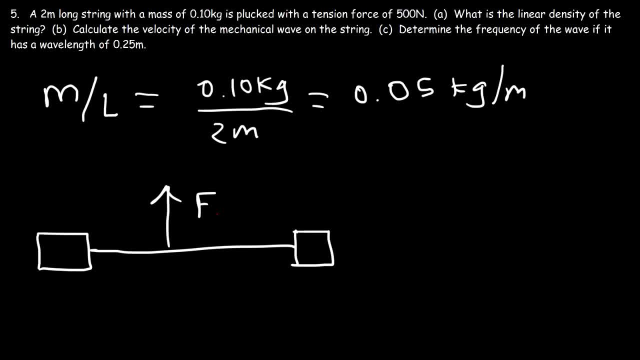 If we apply a force or a tension force on a string, we can create a wave pattern on a string, And so you might get a wave, and what we need to do in Part B is calculate how fast that wave is moving. if we pluck it with a given tension force, the velocity of the wave is equal. 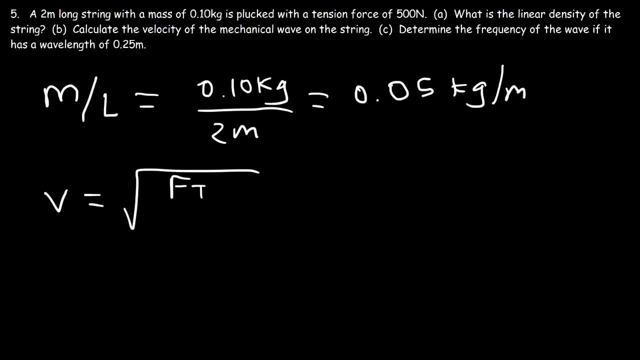 to the square root of the tension force divided by the linear density, the mass per unit left. so in this example the tension force is 500 units and the linear density is 0.05. so 500 divided by 0.05 that's 10,000. if we take the. 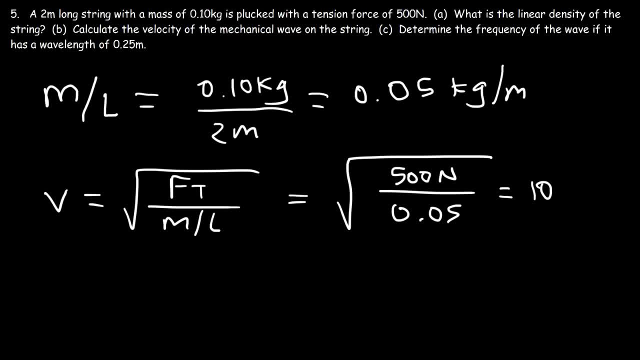 square root of that. that will give us a speed of a hundred meters per second. so that's the answer to Part B. Part C: determine the frequency of the wave if it has a wavelength of 0.25 meters. we know that the wave speed is the. 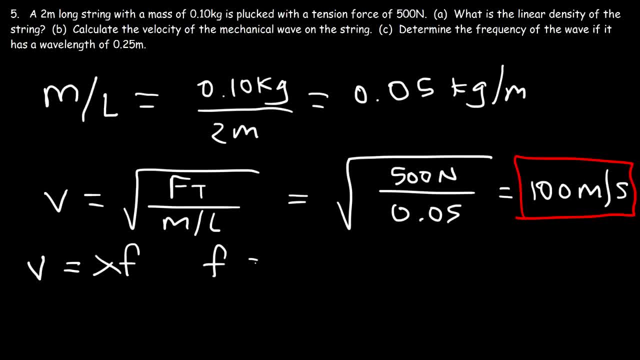 wavelength times the frequency. so the frequency has to be the wave speed divided by the wave length, so it's going to be a hundred meters per second divided by a wavelength of 0.25 meters, and so that's going to give us a frequency of 400 Hertz. and 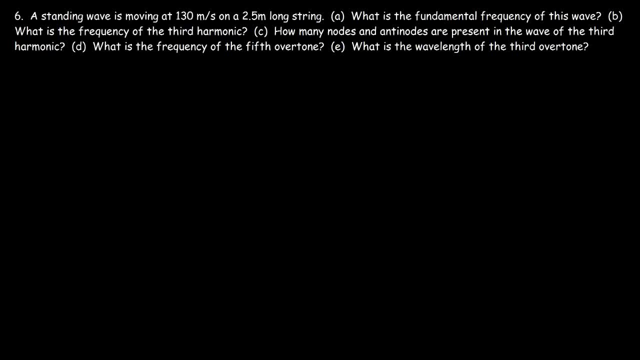 that's the answer to Part C, number six. a standard wave is moving at 130 meters per second on a 2.5 meter long string. what is the fundamental frequency of this wave? feel free to try, if you want to, to calculate the fundamental frequency. you can use this equation. it's. 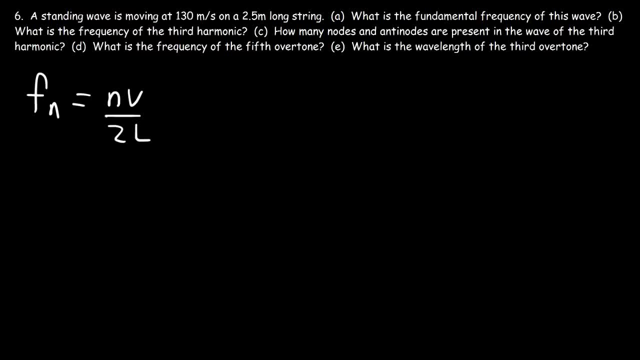 NV over 2L. now N is 1 when dealing with the fundamental frequency, so it's going to be 1 times the wave speed, which is 130 meters per second, and the length of the string is 2.5 meters. so 2 times 2.5 is 5. so it's 130 over 5. so the 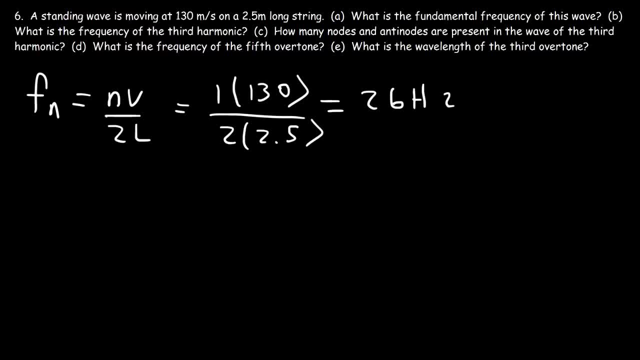 fundamental frequency is 26 Hertz. so that's the answer to Part A. now Part B. what is the frequency of the third harmonic? that's going to be F3. the frequency of the third harmonic is simply three times the fundamental frequency, the fundamental frequency being F1. the second harmonic is F2, the third harmonic F3, fourth harmonic F4, and so 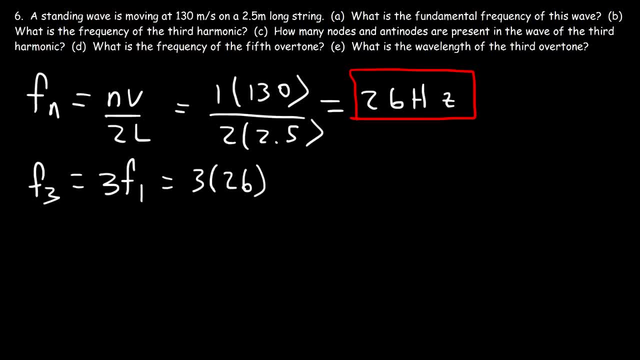 forth. so the third harmonic is simply three times the fundamental frequency, or three times 26, which is 78 Hertz. now let's move on to Part C. how many nodes and antinodes are present in the third, in the wave of the third harmonic? so the first harmonic looks like this: 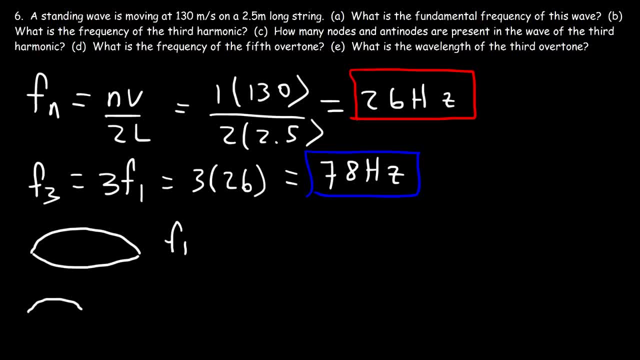 so that's F1. the second harmonic looks like that. that's F2. the third harmonic- let me draw that better. that's the third harmonic. so these are the nodes. the third harmonic has four nodes: the anti nodes or what you have, the maximum displacement, or that's where 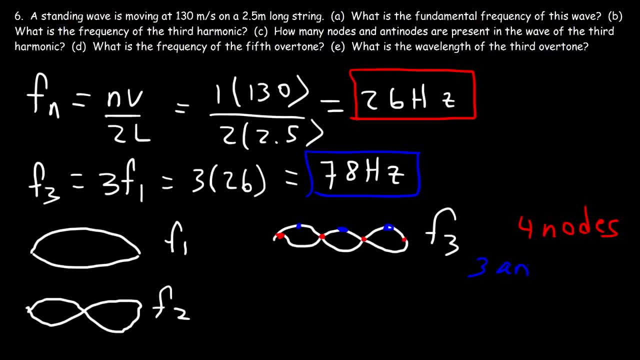 constructive interference occurs. so there's 3 anti notes. the notes occur with destructive interference, that's when the amplitude of the amplitude of the is 0. So the number of nodes is equal to n plus 1, and the number of antinodes is. 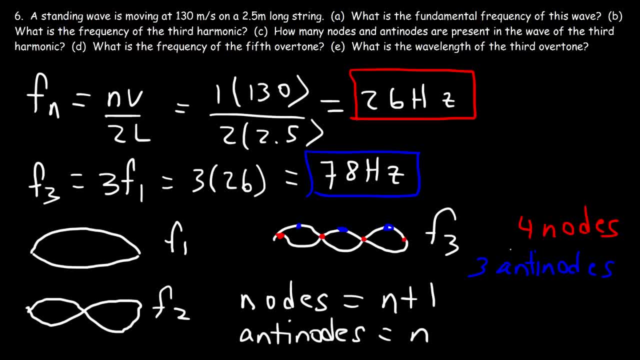 equal to n. So for the third harmonic, n is 3.. Notice that the antinodes and n are the same and the number of nodes is 4, it's n plus 1.. So if we're dealing with the seventh harmonic, the number of nodes is going to be 7 plus 1, it's going to be 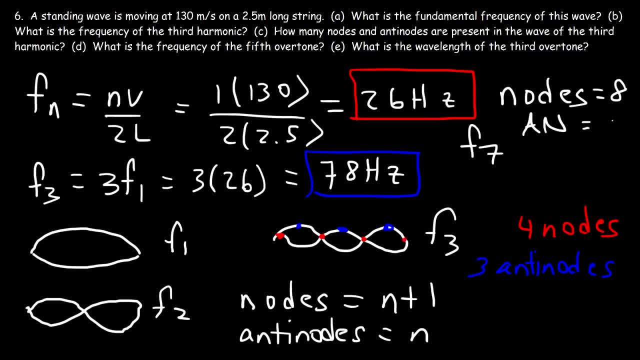 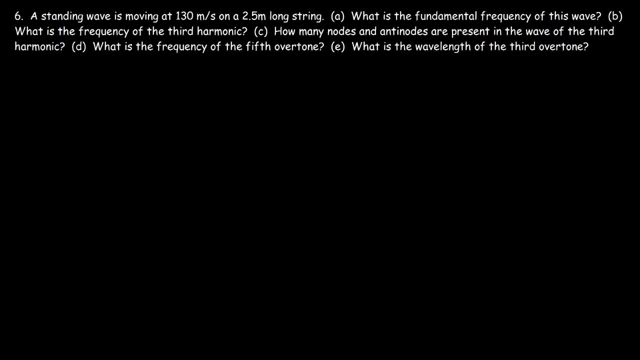 8. The number of antinodes which I'm going to denote a n, that's going to be 7.. Now let's move on to part D. What is the frequency of the fifth overtone? You need to know that the first overtone- I'm just going to put ot for overtone, the first. 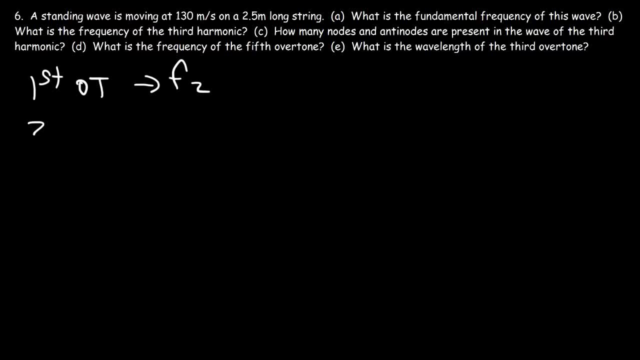 overtone corresponds to the second harmonic, The second overtone corresponds to the third harmonic. So the fifth overtone corresponds to the second harmonic. So the fifth overtone corresponds to the sixth overtone corresponds to the sixth overtone, and the sixth overtone corresponds to.